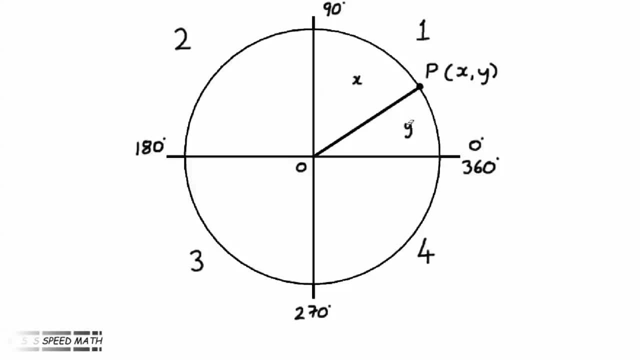 a radius to the circle, Rotating the radius about the origin in an anti-clockwise fashion. you can see our angles of increasing value are swept out all the way to 360 degrees. We will be looking at an angle theta. The angle theta is the radius of the point P as it increases in value from one quadrant. 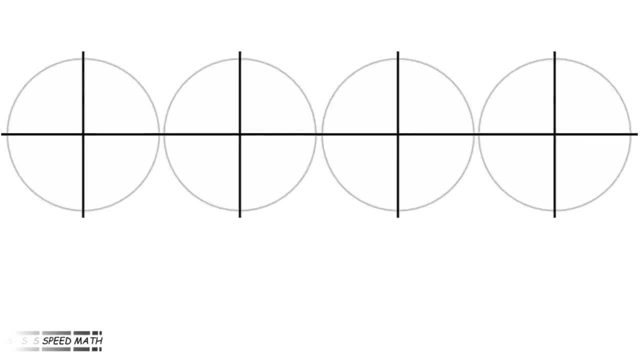 to the next. The value of the trig functions sine cosine and tangent are gleaned from the xy values of the point P and the radius length, which is 1.. So straight away, looking in the first quadrant, at the triangle made by the radius, which is: 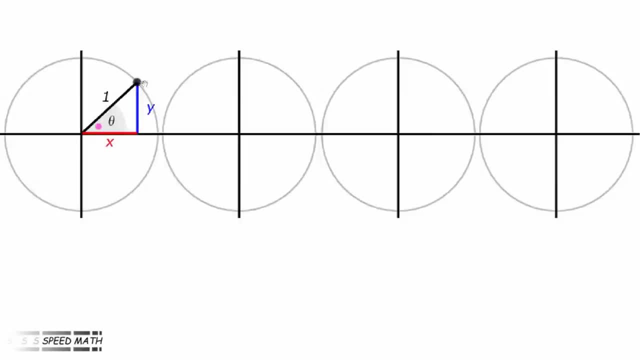 the hypotenuse and the sides x and y, you can see that sine theta equals y over 1, cosine equals x over 1 and tan theta equals y over x. Now, since in this quadrant, quadrant 1, both x and y are positive, sine theta, cosine theta and tan theta are all positive, 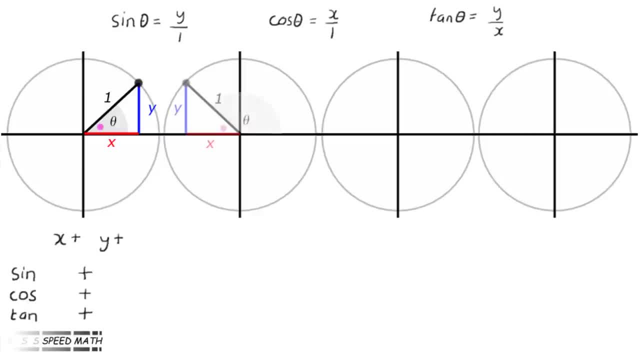 Looking at the second diagram, if we rotate the radius around a bit further, so it sits in quadrant 2, the angle it represents is somewhere between 90 and 180 degrees. x is negative and y is positive, so here sine theta is plus y over 1,, therefore positive. 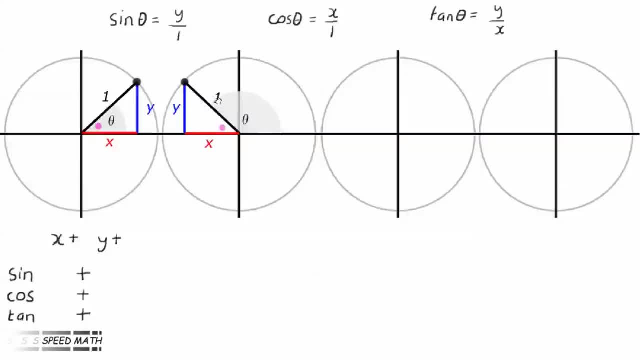 Cosine theta is minus x over 1,, therefore negative. Tan theta is plus y over minus x, therefore negative. Now looking at the third diagram, if we rotate the radius around a bit further still, so it sits in quadrant 3,. 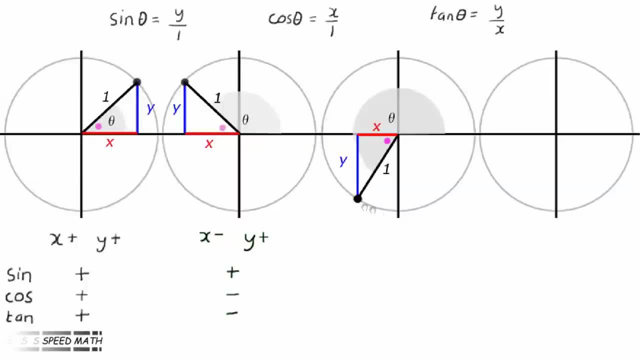 the angle it represents is somewhere between 180 and 270 degrees. x is negative and y is negative, so sine theta is minus y over 1, therefore negative. Cosine theta is minus x over 1, therefore negative. Tan theta is minus y over minus x, therefore positive. 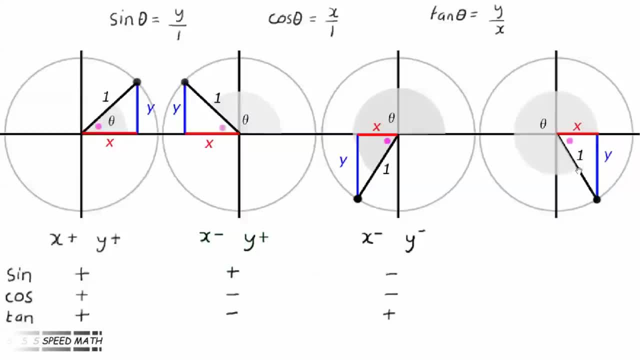 Looking at the fourth diagram, if we rotate the radius around still further, tan theta is minus y over minus x, therefore negative. If we rotate the radius around still further, tan theta is minus y over minus x, therefore negative. If we rotate the radius around still further, tan theta is minus y over minus x. therefore, 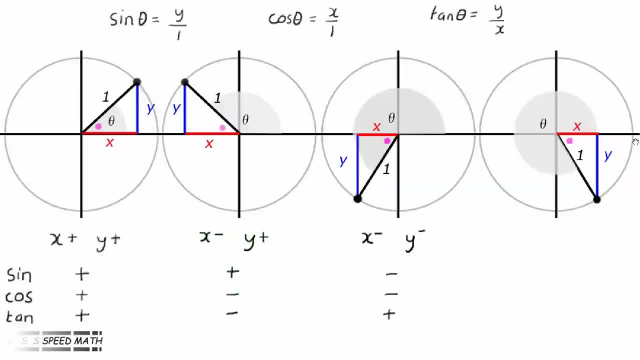 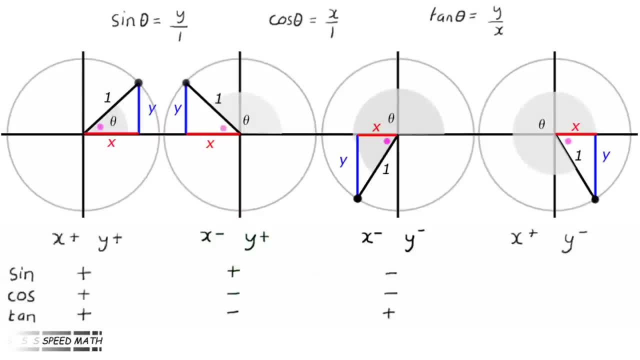 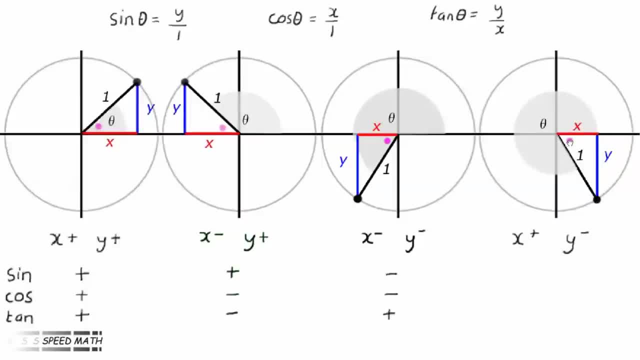 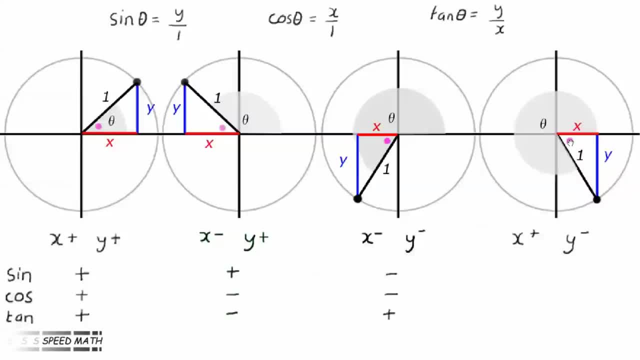 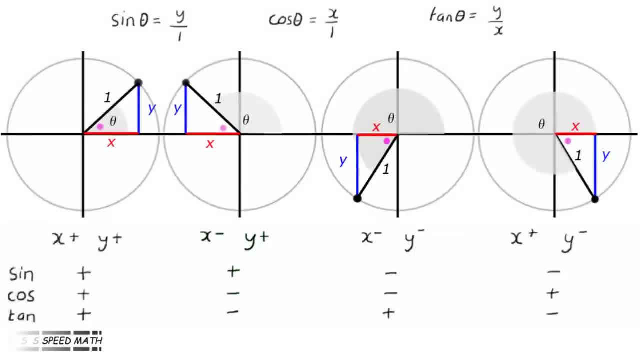 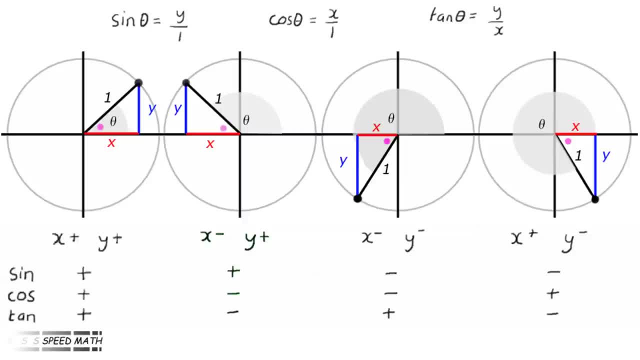 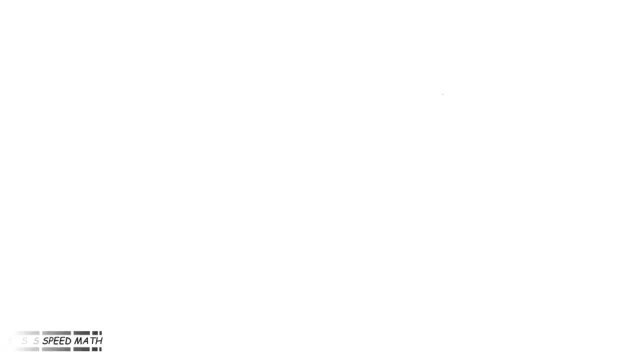 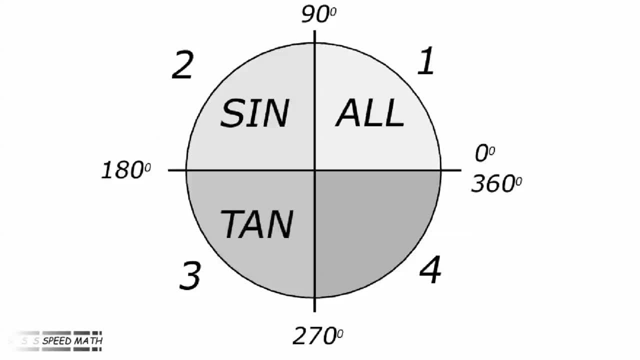 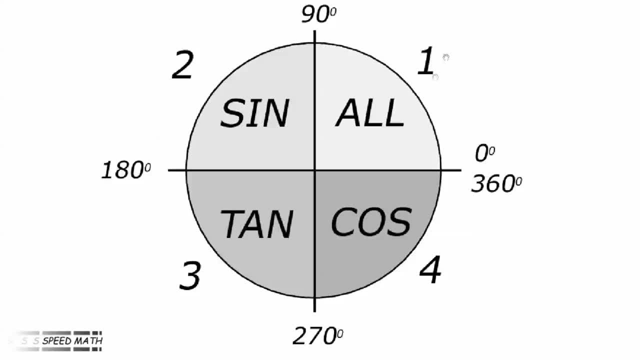 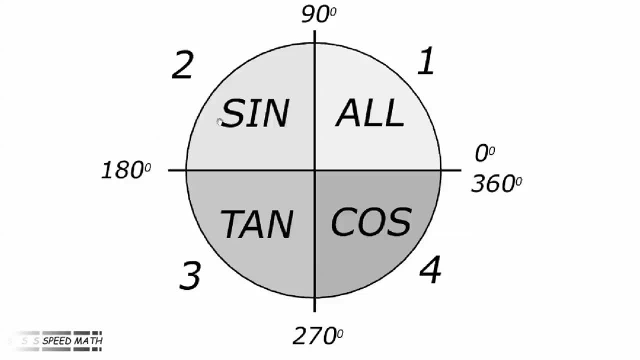 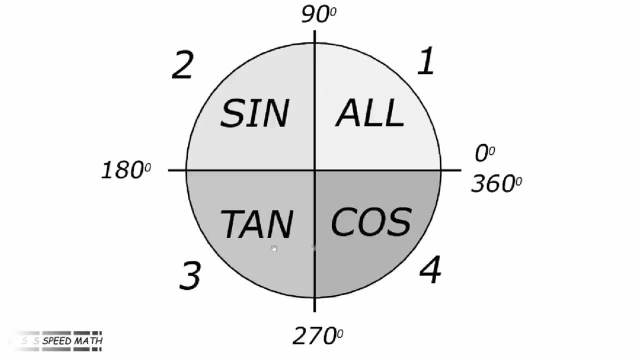 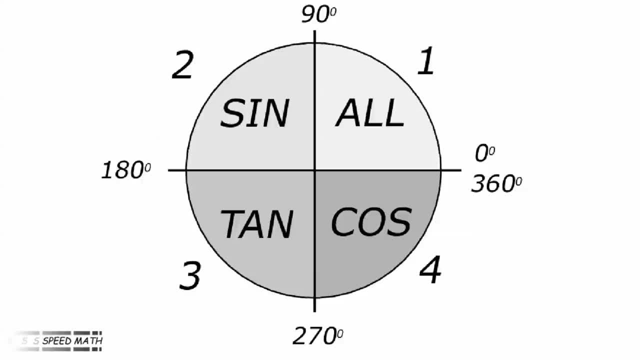 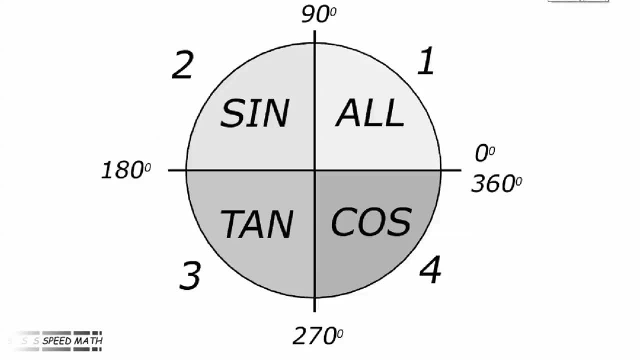 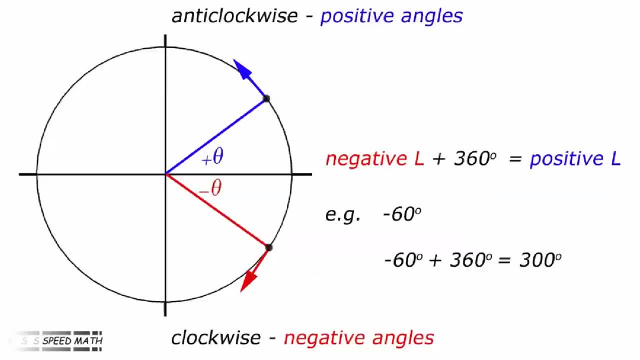 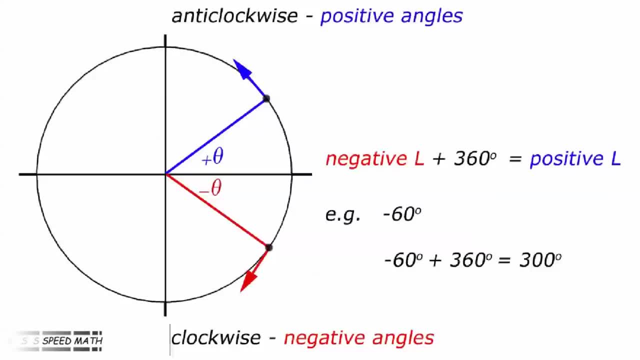 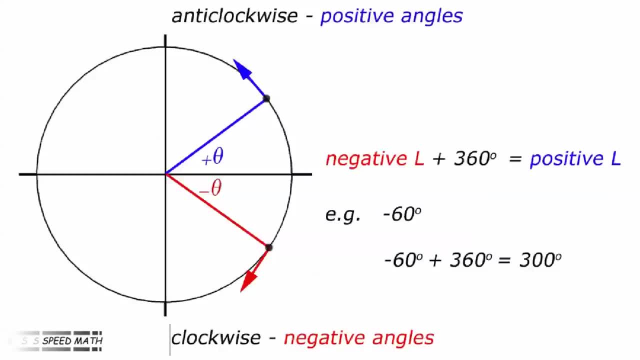 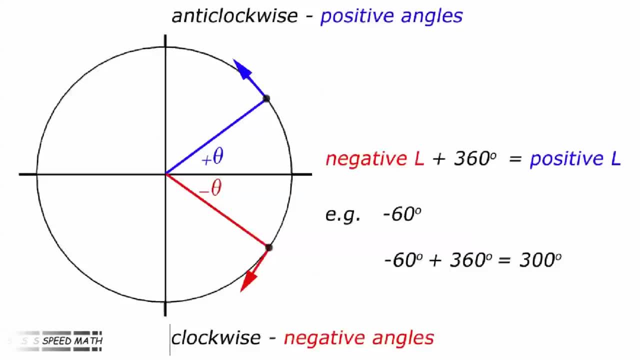 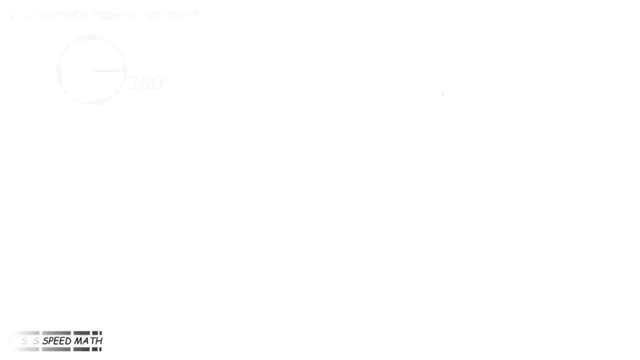 negative If we rotate the radius around still further. tan theta is minus y over minus x. therefore degrees, and we just take it from there, your calculator will do the rest. very large angles are those greater than 360 degrees, in other words greater than one rotation. such angles are 565. 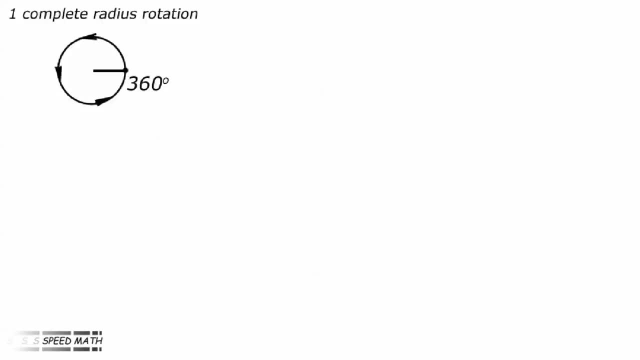 degrees, 750 degrees, 1200 degrees. we can easily bring these down to size by taking away 360 degrees until we get a remainder that is less than 360.. so 565 degrees is the same as 565 minus 360, which is 205 degrees. 750 degrees minus 360 degrees gives us 390 degrees. 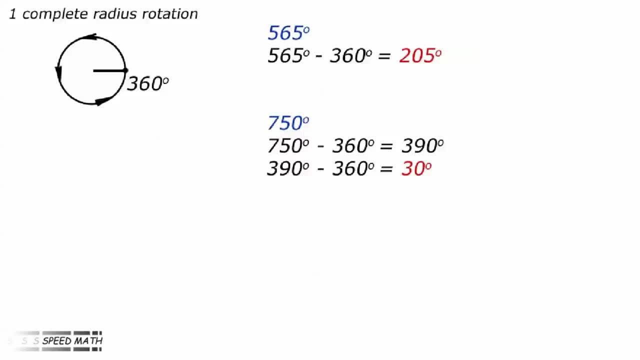 if we take another 360 away, we get 390 minus 360, which equals 30 degrees. 1200 degrees minus 360 degrees is 840 degrees. taking away another 360 degrees, we get 480 degrees, and taking away yet another 360 degrees, we get our final answer of 120 degrees. 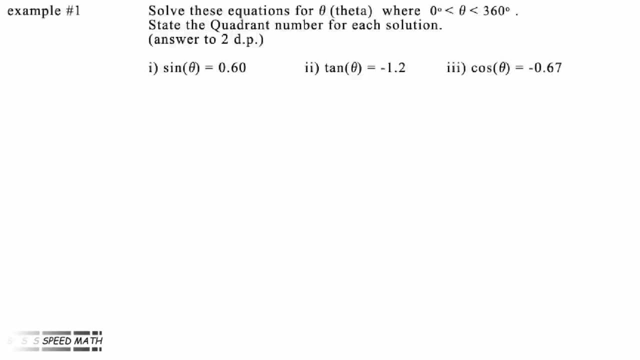 and now to the problems. example number one: solve these equations for theta. where theta is greater than zero degrees and less than 360 degrees, state the quadratic number for each solution. answer to two decimal places: one sine theta equals 0.60. two tan theta equals minus 1.2. 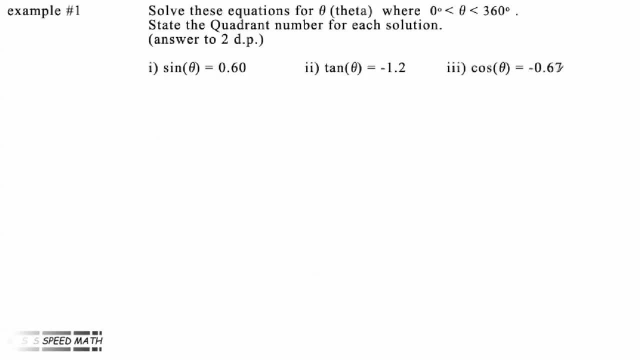 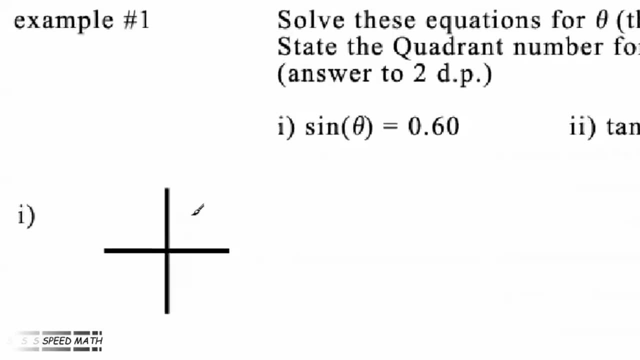 number three, cosine theta equals minus 0.67.. The first thing we need to do is to visualize the problem. So we start with our axes and the angles anti-clockwise, from zero degrees, 90,, 180,, 270, and 360 degrees. 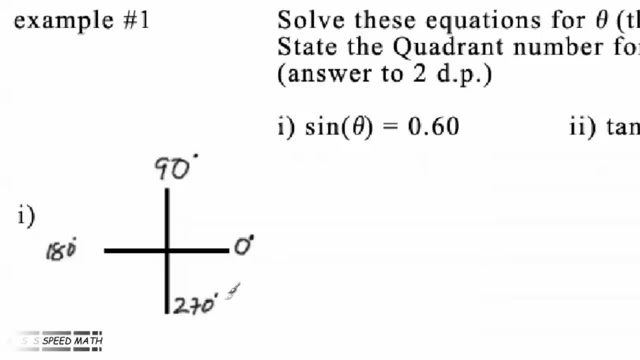 or back to zero. I label the four quadrants- one, two, three, four- anti-clockwise. The angle of theta has a positive sign, So it lies as an acute angle in the first quadrant, But a positive sign also corresponds. 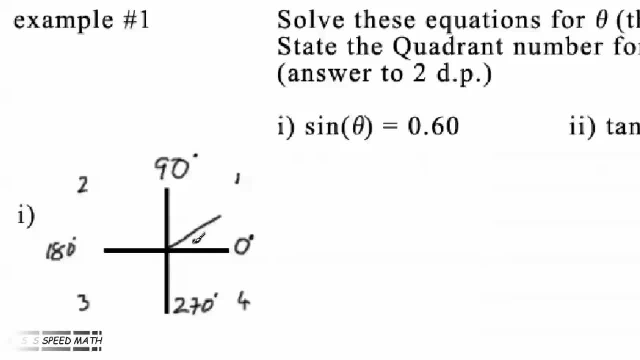 to an obtuse angle in the second quadrant. The supplementary angle- the one, when added to the obtuse angle, makes 180 degrees- is the mirror of our acute angle in the y-axis. The second thing we need to do is to find the angle of theta in the y-axis. 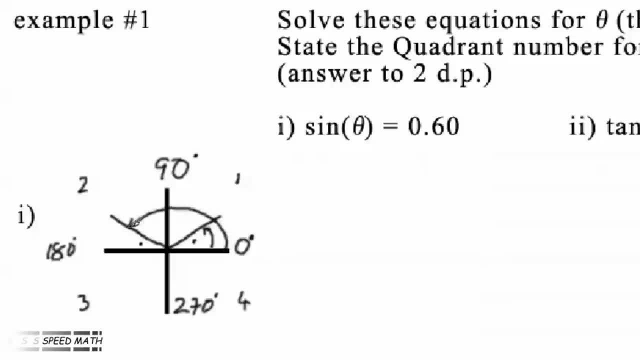 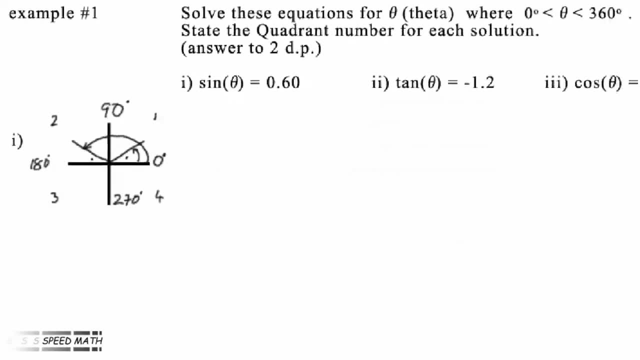 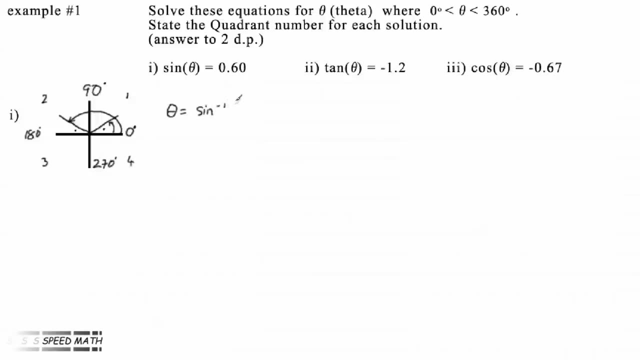 So to find that obtuse angle, all we have to do is take the acute angle away from 180 degrees. Okay, so let's find theta. Theta is equal to sine minus one of 0.60. And this comes to an angle of 36.2 degrees. 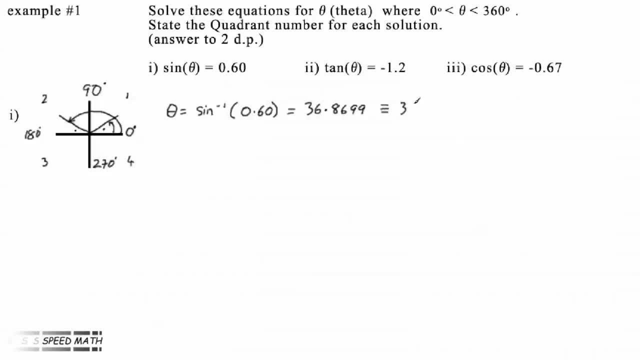 It's equal to 0.8699 degrees, which is equivalent to 36.87 degrees to two decimal places. Yeah, this is in the first quadrant. Okay, the other solution, where sine theta is positive, is in the second quadrant. 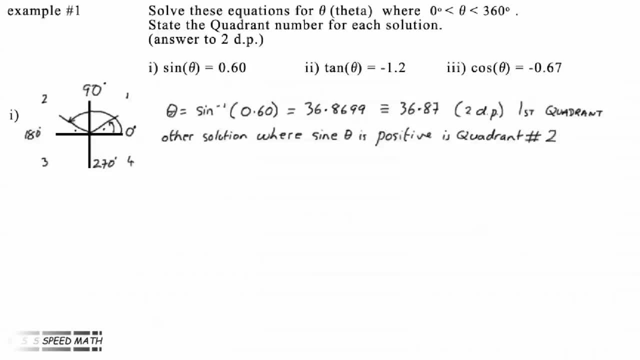 So we can write: theta is equal to 180 degrees minus 36.87 degrees, which is equal to 143.13 degrees. So here are our solutions. This is the first quadrant. The second is negative. our solutions: 36.87 degrees. first quadrant, 143.13 degrees. the second quadrant: As before. 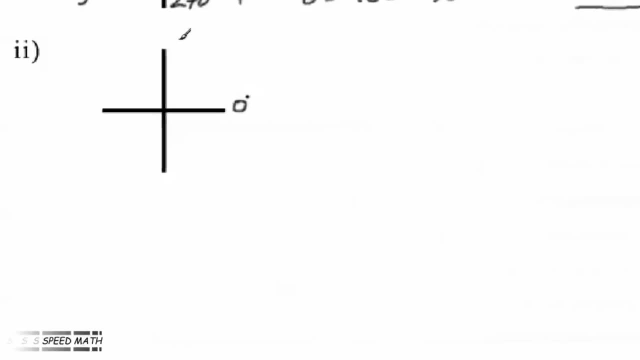 we start with our axes, angles and quadrants 0,, 90 degrees, 180 degrees, 270 degrees, 260 degrees and quadrants 1,, 2,, 3 and 4.. Now, if we choose the tan minus 1 function on our calculator, 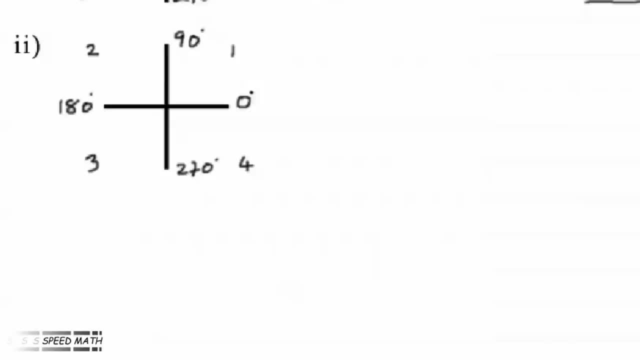 and type in minus 1.2, we get the angle minus 50.1944 degrees, which is minus 50.19 degrees to two decimal places. This angle is outside of a range. The question stipulates that theta must be between 0 and 360 degrees. Now, tan theta is only negative in the second and fourth quadrants. 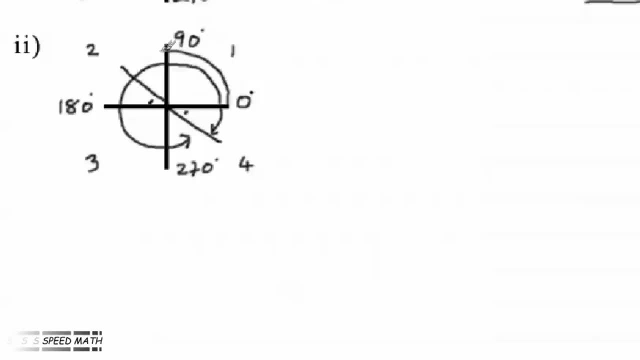 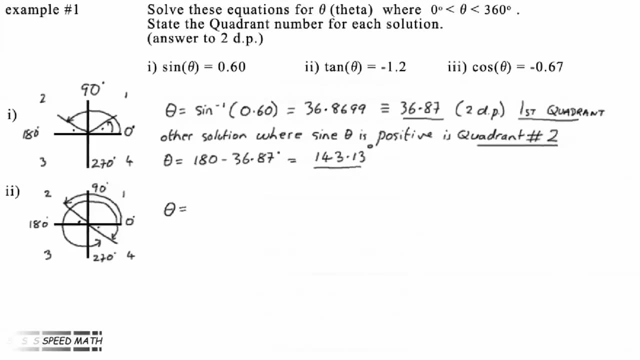 so the angle must be a reflex angle in quadrant 4 and an obtuse angle in quadrant 2.. Writing this down: theta equals tan minus 1 minus 1.2. so theta is equal to minus 50.1944, which is minus 50.19 to two decimal places Quadrant 2. 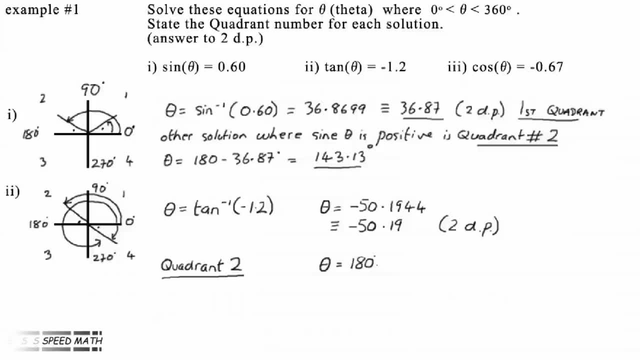 we have, theta is equal to 180 degrees minus 50.194 degrees, which makes theta equal to 129.81 degrees. In quadrant 4, theta equals 360 degrees minus 50.19 degrees, which makes theta equal to 309.81 degrees. 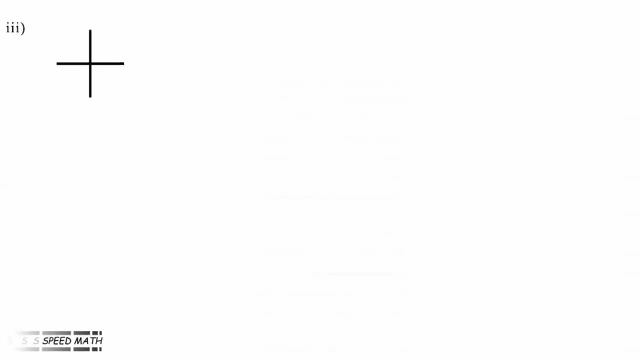 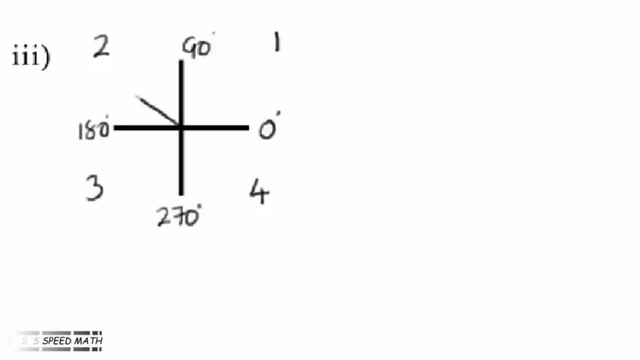 one function on our calculator and type in minus 0.67, we get the angle 132.0671 degrees, which is 132.07 degrees to two decimal places. this angle is clearly in quadrant two. now cosine theta is only negative in the second and third quadrants, so the angle must be an obtuse angle in quadrant. 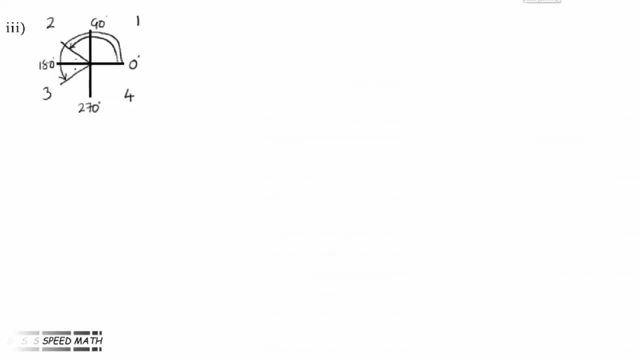 two and a reflex angle in quadrant three. okay, writing all this down, we have: theta is equal to cosine minus one minus 0.67 and that's equal to 132.0671 degrees, which makes theta equal to 132.07 degrees to two decimal places. okay, that's in quadrant two. so 132.07 degrees in quadrant two. 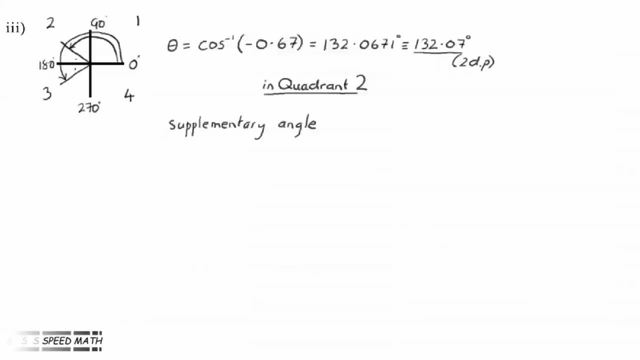 okay, the supplementary angle is equal to 180 degrees minus 132.07 degrees, which makes the supplementary angle to 47.93 degrees. okay, in quadrant three we have: theta is equal to 180 degrees plus 47.93 degrees, which makes theta equal to 227.93 degrees. 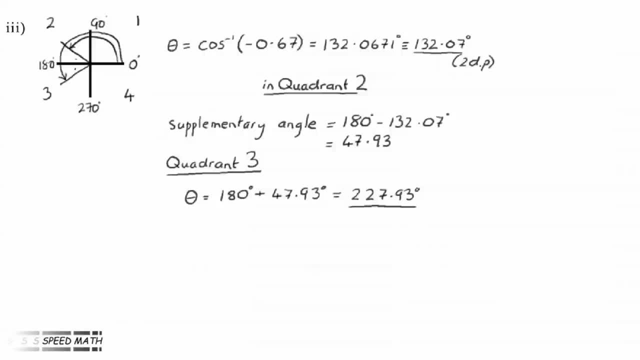 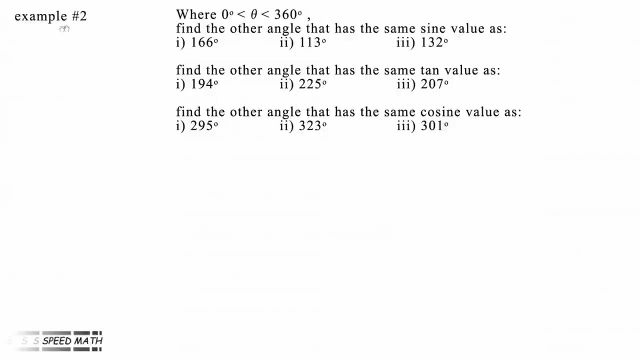 example number two, where theta is between 0 and 360 degrees. find the other angle that is the same sine value as 166, 113, 132 degrees. find the other angle that has the same tan value as 194, 225, 207 degrees. find the other angle that is the same cosine value as 295, 323 and 301 degrees. 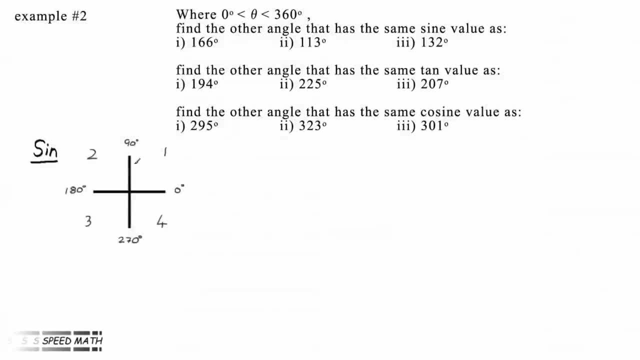 you'll notice that all these angles in the first part of the question are in the second quadrant. their sine values are all positive- remember all sine tan cos- and they have the very same values as their supplementary angles, that is, the angles that they make up 180 degrees with. looking at the diagram, the supplementary angle is the mirror image of 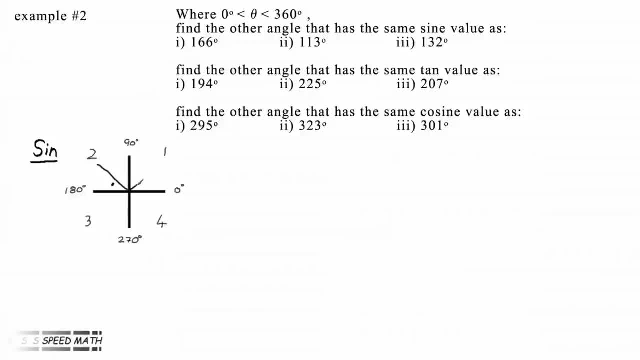 the acute angle in the first quadrant. to calculate the value of the acute angle, all we have to do is subtract the obtuse angle from 180 degrees. so our required angles are: first one: 180 minus 166 equals 14 degrees. second: 180 minus 113 equals 67 degrees. third one: 180 degrees minus 132 degrees. 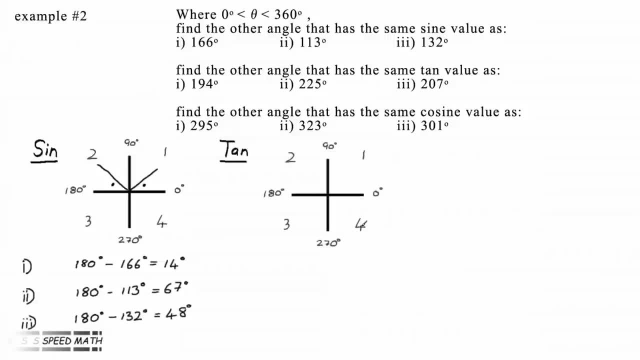 equals 48 degrees. you will notice that all these angles in the second part of the question are reflex and in the third quadrant their tan values are all positive in this quadrant. remember, all the angles are positive in this quadrant and all the angles are positive in this quadrant. 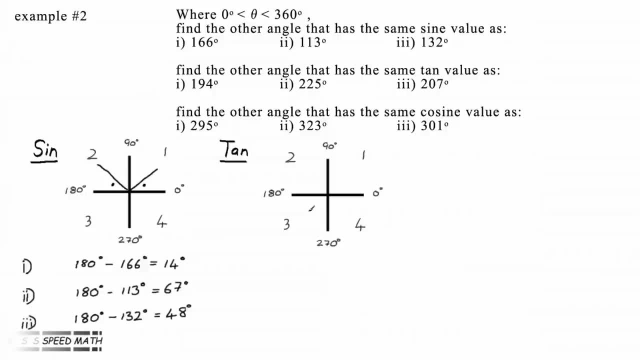 sine tan cos, and they have the very same values as the acute angles in quadrant one. looking at the diagram, the acute angle that the radius makes with the x-axis is vertically opposite to the acute angle in the first quadrant. so in order to calculate the value of the acute angle, all we have to do is: 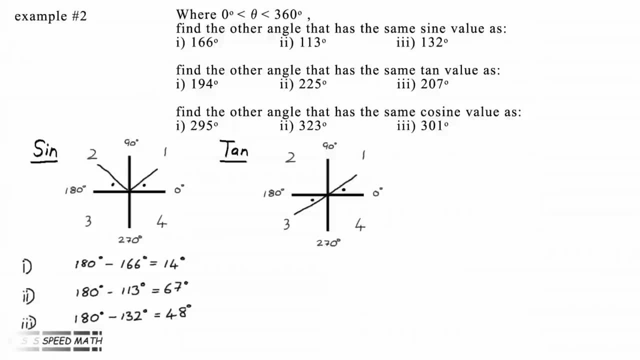 subtract a hundred and eighty degrees from the angle, so our required angles are one, 194 minus 180 equals 14 degrees. to 225 minus 180 degrees equals 45 degrees. and three, 207 minus 180 equals 27 degrees. you'll notice that all these 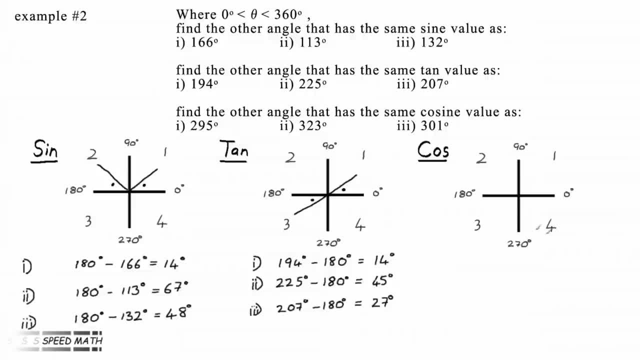 angles in the third part of the question are reflex and in the fourth quadrant. this time, their cosine values are all positive in this quadrant, remember all sine tan cos and they have the very same values as the acute angles in quadrant one. looking at the fourth quadrant, the 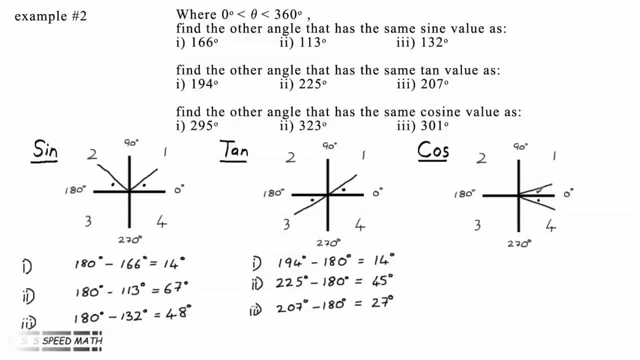 acute angle that the radius makes with the x-axis is a mirror image of the acute angle in the first quadrant. so in order to calculate the value of the acute angle, all we have to do is subtract the reflex angle from 360 degrees. so our required angles are one, 360 minus 295, which gives us 65 degrees. 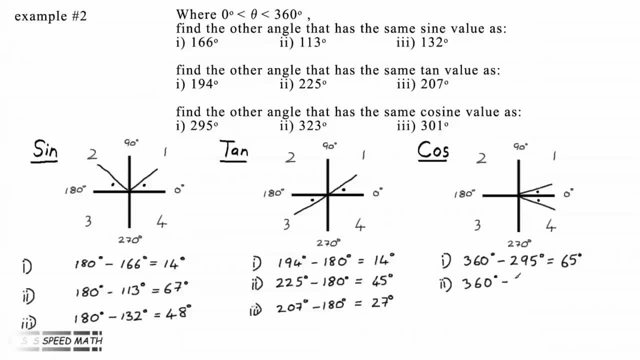 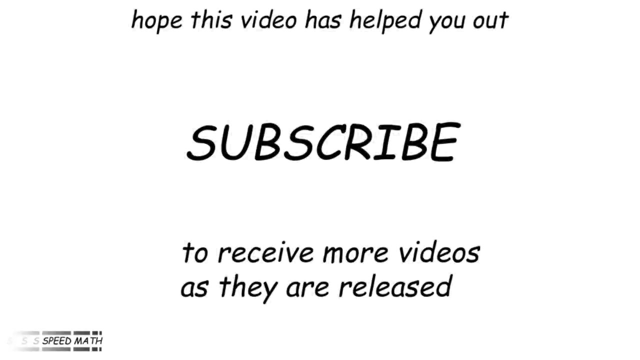 to 360 minus 323 degrees equals 37 degrees, and three 360 minus 301 gives us 59 degrees. and that's all, folks. in fact, that is all for this particular series, basic trig, but don't despair, there will be other topics coming soon. anyway, thank you all. 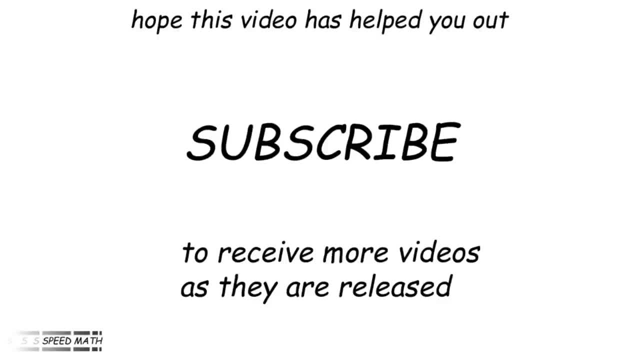 for watching. please do subscribe to the channel and be the first to see all the latest releases. see you soon. you.